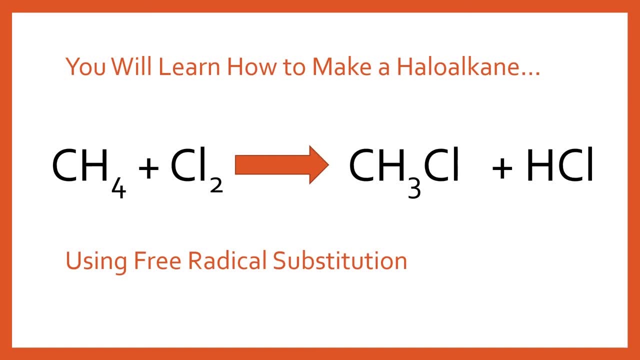 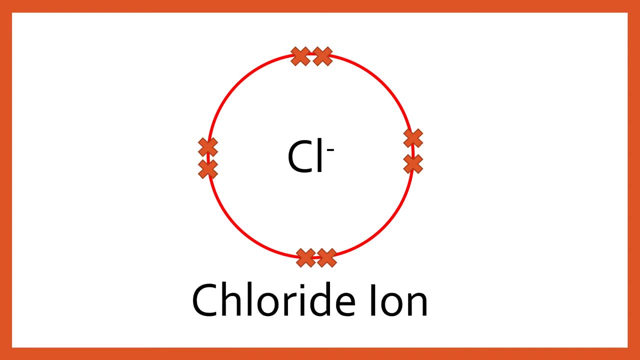 But before you can actually understand this reaction, you have to understand some keywords. So the first one is to understand the concept of an ion. So here we have a substance that's called a chloride ion, and chlorine is in group 7. It's got an extra electron in its outer shell. It's now stable. 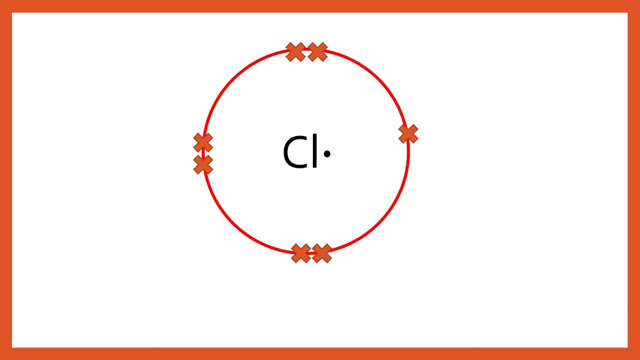 However, if it were to lose one like this, it becomes something called a chloride. It's called a chloride radical, and this radical is extremely reactive And we show the radical by simply putting a dot outside of it, and that's representing an electron that is unbonded. 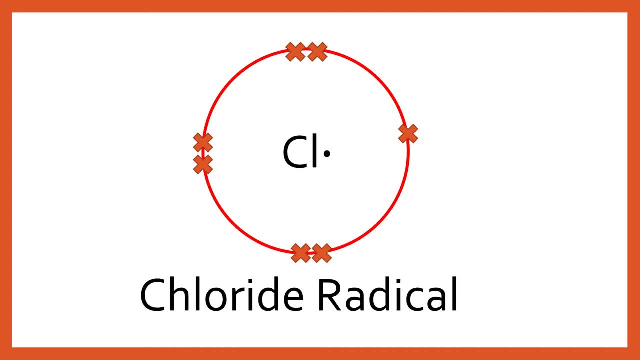 This chlorine is likely to be extraordinarily reactive with most things and will try and form another bond in order to get back to that stable structure. The next set of keywords that you need to understand are for understanding the steps in free radical substitution, And the first one is initiation, and that means starting off the reaction. 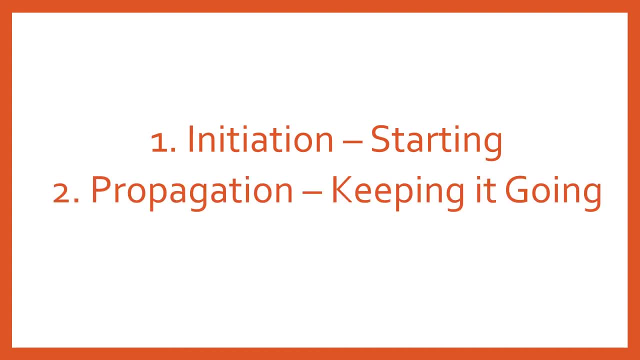 If you initiate something, it means to start something. Then you've got propagation as the next stage and that's keeping it going. It's propagating the reaction And then at the end, unsurprisingly, we have termination. So it means stopping the reaction. 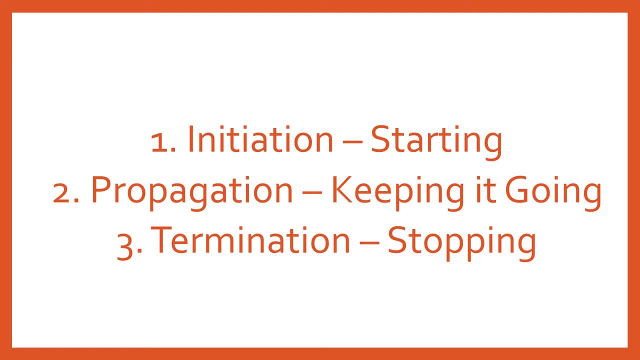 So it goes through three steps: starts with initiation at the beginning, works through some propagation steps and then you have some termination that stops the reaction from happening and ends the process. And we will run through all of these. So let's take a look at some of the steps in understanding how the free radical substitution works. 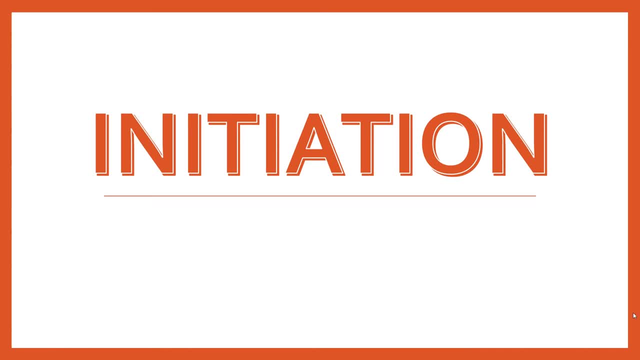 So let's start by looking at initiation And, as I've said previously, initiation is all about getting the reaction started. So here we have Cl2.. And, as you can imagine, Cl2 is not going to be wildly reactive. So what's going to have to happen to make it actually react is that that bond is going to have to be broken. 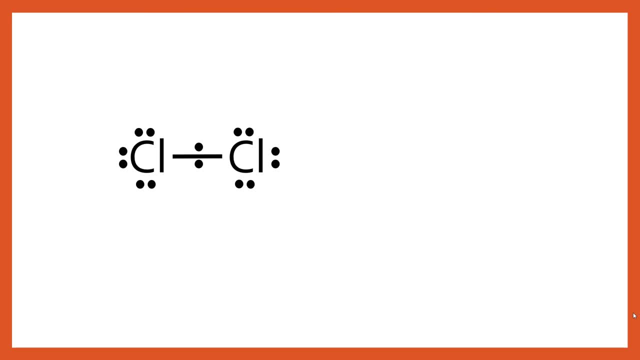 And so I've shown all of the electrons as dots and we've got a line for the bonds. Now we need that bond to be broken And we need to have some energy input in order to break it. So we have some UV radiation, some high energy radiation that is able to break that bond. 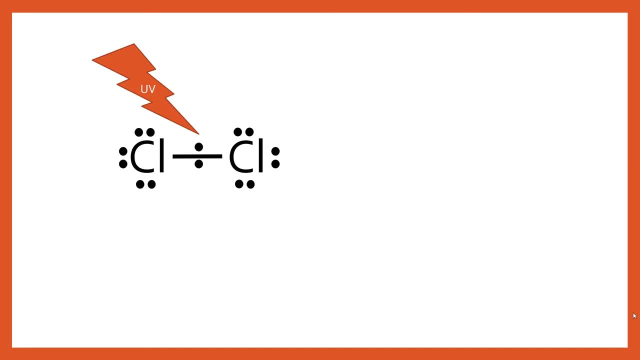 And when the bond breaks, the electrons are going to move in a very specific way. They're going to move like this. So one chlorine is gaining one electron, another chlorine is gaining another electron. So in other words, both of the two Cls are getting the same number of electrons. 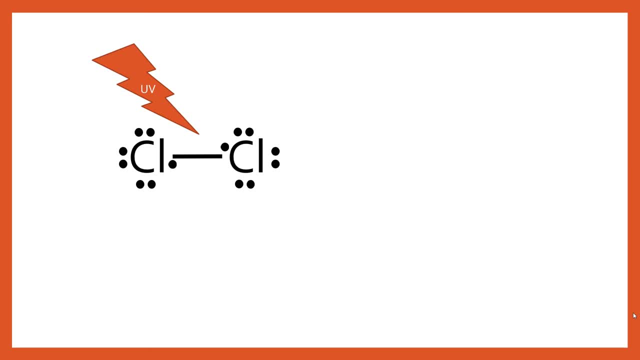 So this is sometimes called homolytic fission, Homo meaning same homolytic fission where the word fission is to do with splitting up. We have homolytic fission of the bond. Each Cl species is getting the same number of electrons and the bond is breaking. 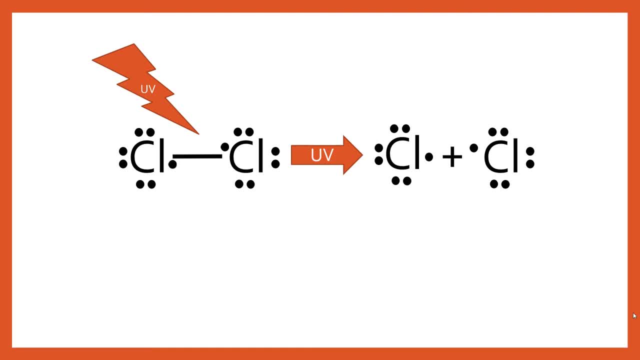 And this will give rise to two free radicals. So you can see that both of those chlorines is like the radical I showed you before. They're going to be hugely reactive as they have an unbonded electron that would like to find another electron to form a covalent bond. 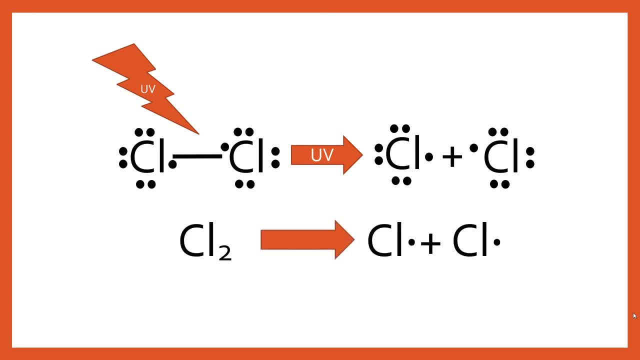 So we can write this in a simpler form. We can just say Cl2 becomes and then show the two radicals that it is forming. This is going to get the reaction started, because we've started with that unreactive Cl2 that is, of course, quite stable. 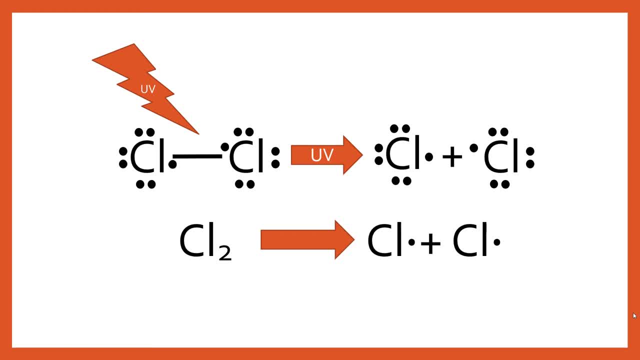 It's got the full outer electron shell with the covalent bonds, whereas now it is two free radical species that are extremely reactive and they are going to start breaking up some other substances and get the reaction going, And so that brings us to propagation. 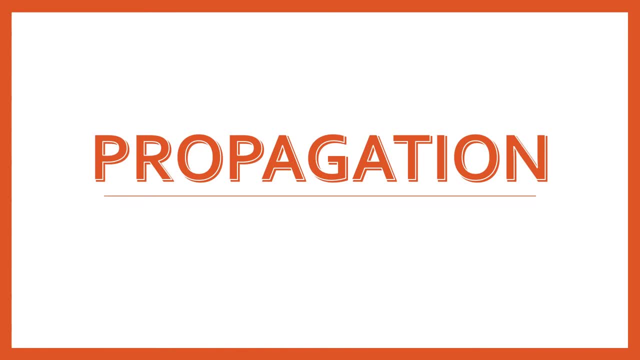 What's going to get this reaction going? And for this particular reaction, we're going to have multiple different propagation steps And I'm going to explain each of these in turn. So let's start by reminding ourselves of the fundamentals. So we're looking at this reaction and I've highlighted two of these in bold. 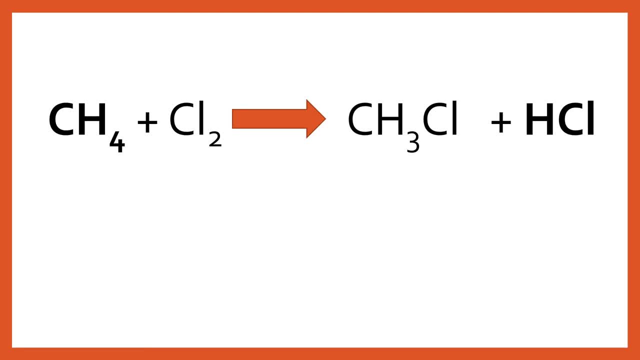 So we're going to look at how the CH4 reacts and how the HCl is actually formed. We've also seen previously that we've got an initiation step where we're getting two chlorine radicals formed, And so let's look at what would happen. 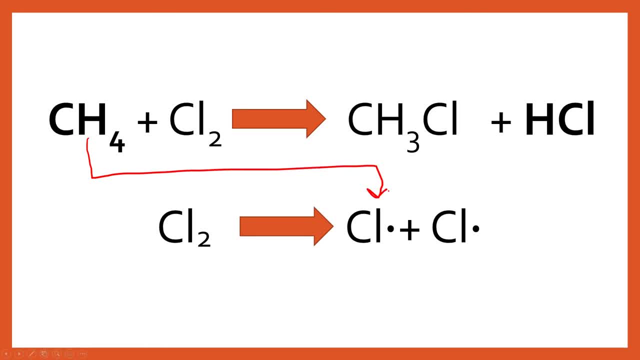 If one of our CH4s was to react with one of the chlorine radicals. So let's take our CH4 and draw it out in full, showing all the electrons and the bonds, And if we were to react it with a radical, we'll see a kind of movement and rearrangement in the electrons. 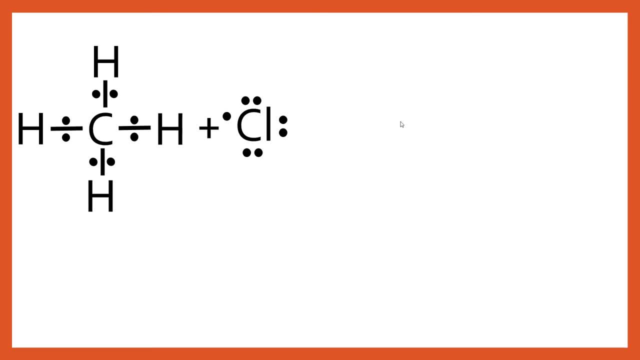 So you've maybe seen previously about curly arrows that show the movement of a pair of electrons. We can show the movement of single electrons with a kind of half arrow. So let's perhaps look at this electron and have it go to the carbon, And then this electron is going to come into this space in here. 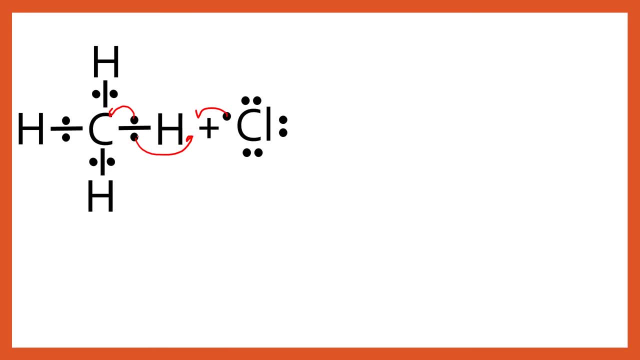 And then this one's going to go like this: So this electron and this electron are going to form a bond, So the hydrogen and chlorine are going to join together, And then one of these electrons is going to go back to the carbon, So we've got homolytic fission and this is going to become CH3. 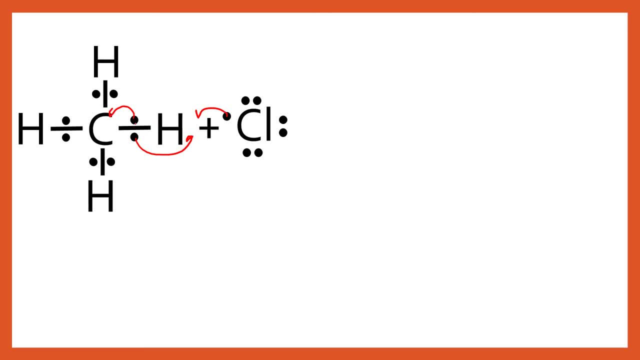 when the bond breaks and the hydrogen goes off, And it's going to be a radical because it's got one electron going back, And then you're going to get a covalent bond forming with this electron and this electron forming a pair of electrons. 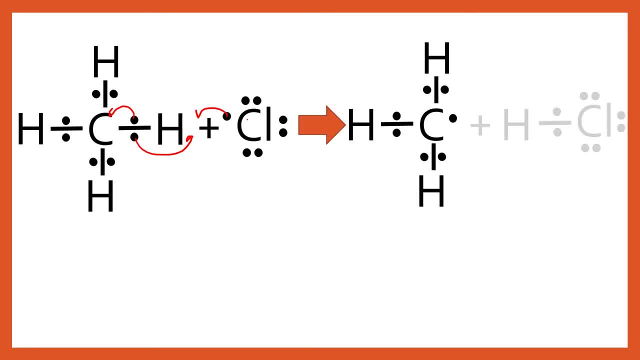 So you'll get the hydrogen bonding to the chlorine. So there's your first product and there's your second product. So we can write this more succinctly as so? So we can just have CH4 for the methane Cl dot showing that radical. 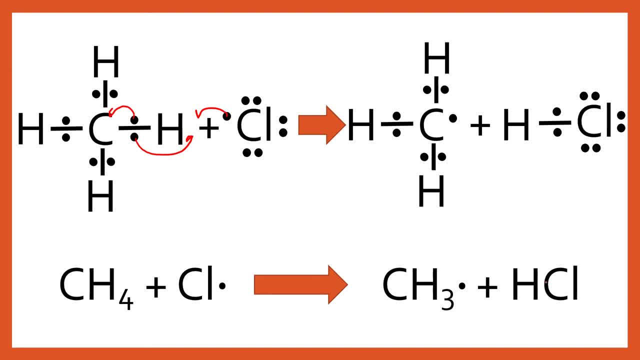 And now we're getting a CH3 radical with an HCl. So what you must notice here is that we're starting with a CH4, which is stable, reacting it with a radical, forming another radical and then forming a stable product. So we've got this CH3 radical. 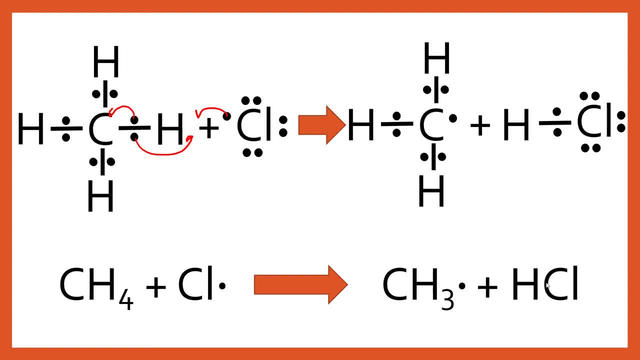 That's going to be extremely reactive and that could react with some other things. So let's carry that CH3 forward and look at what happens to that. So here we have a CH3 and it's a radical And you can see that with the dot that's on its own. 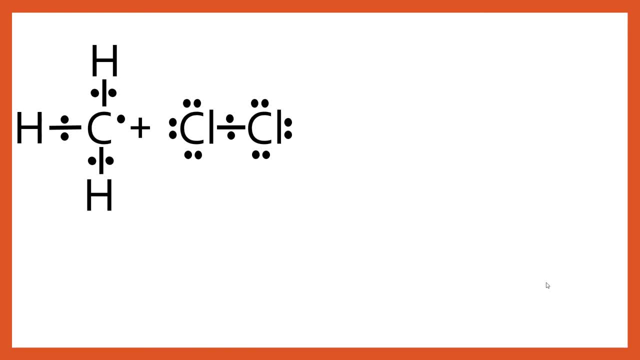 That could react with, let's say, some Cl2 that's not been split up by the UV, So we've got that simple Cl2.. Now, when this reacts, we get this product. So basically, what's happening is one of the chlorines is breaking off. 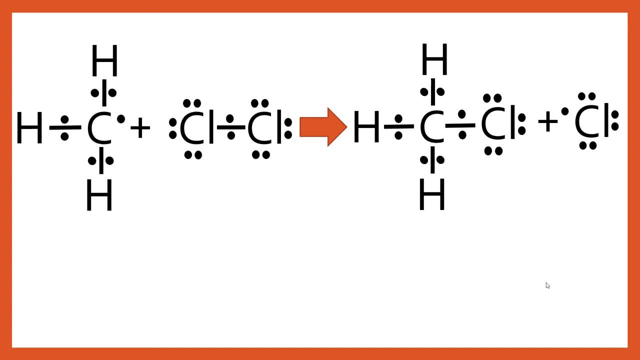 and is now a radical, And one of the chlorines is being joined to the CH3. And again, what you should see happening is that we had a radical react with a non-radical species to form a non-radical species and then another radical comes back. 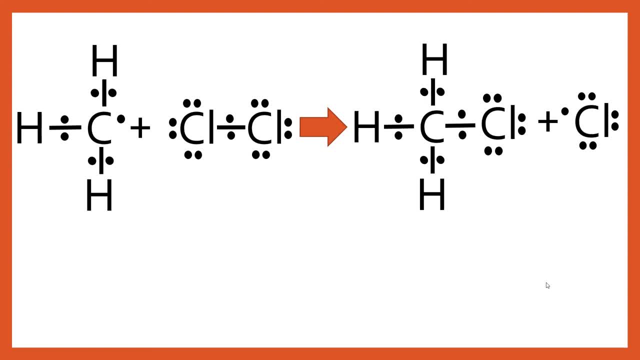 We just got rid of that Cl. that Cl radical got rid of last time and now it's come back again. So this Cl is going to start reacting with some other stuff. So it's propagating the reaction. Yes, we're getting rid of one radical. 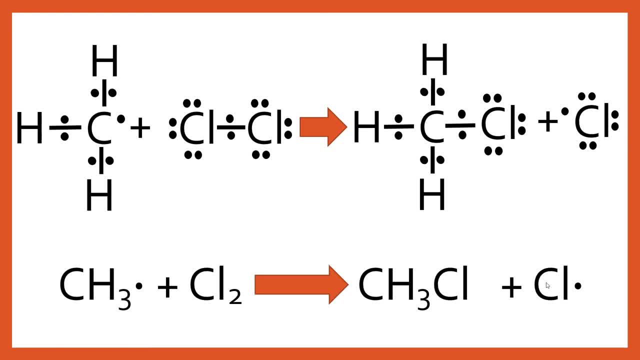 species, but then making another one. that's what's propagating the reaction. And we can write this again succinctly: with the CH3 radical plus the chlorine gas, There's our desired product, the synthesis of a halo alkane, which was the intent. 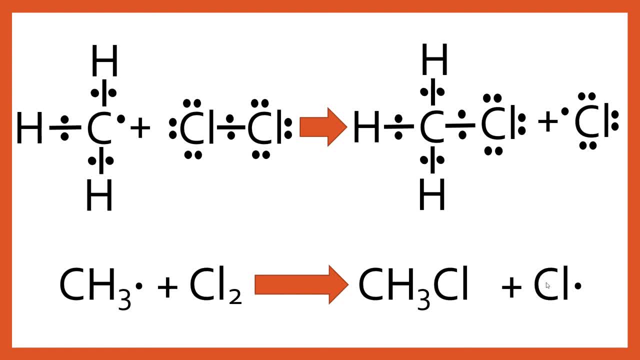 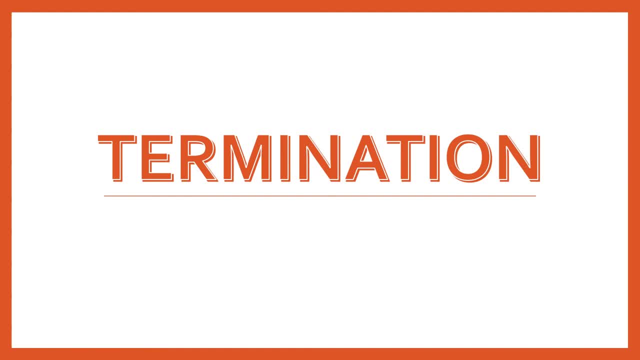 But we're also getting this radical that's going to start reacting with some other stuff and just keep things going. So let's look at what happens next, which is termination. Termination is really all about putting a stop to it, Taking those radical species and essentially soaking them up and forming. 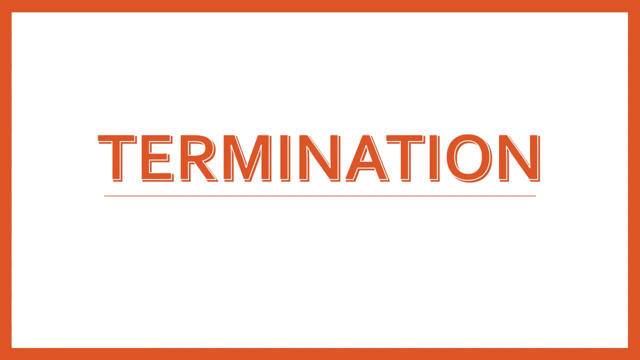 stable products that are taking away those radicals and ending the reaction. And there's various ways in which this can happen. So, for example, we've seen the initiation reaction where the chlorine is broken up to produce two radicals- The most simple and obvious termination. 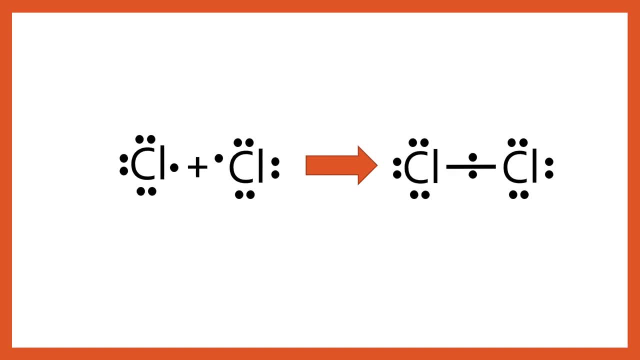 step is to just take this equation and write it backwards. So we have two radicals reacting together, forming Cl2 again. The Cl2 is, of course, a stable product, So you're ending up with basically reversing the initiation step for a termination reaction. 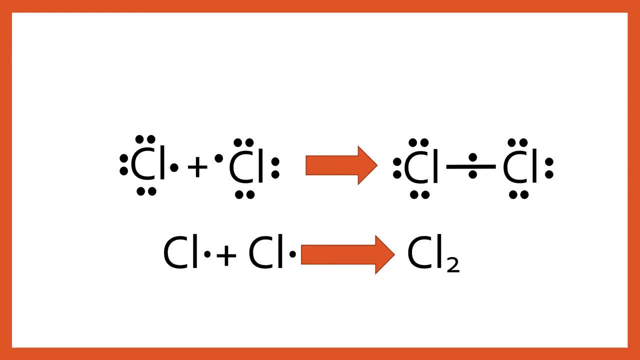 So that is the simplest one. We have some other ones that we can look at in a second. We can also represent that more simply with that equation there. So let's look at the other possible reactions. We could have two of the CH3 radicals finding each other, and then they could. 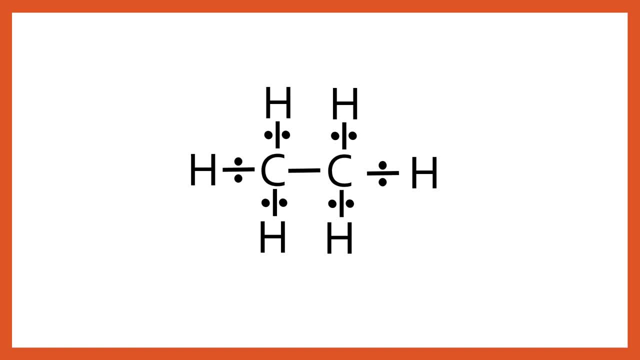 just join together something like this: form a covalent bond, And there you're going to get a stable product, And so that's going to look like this: You've got a CH3 and a CH3, both of which are radical, simply forming C2H6. 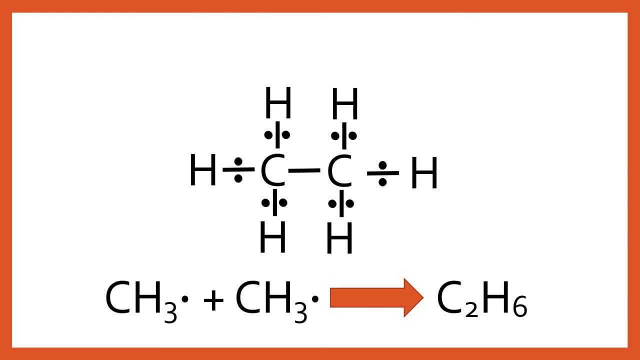 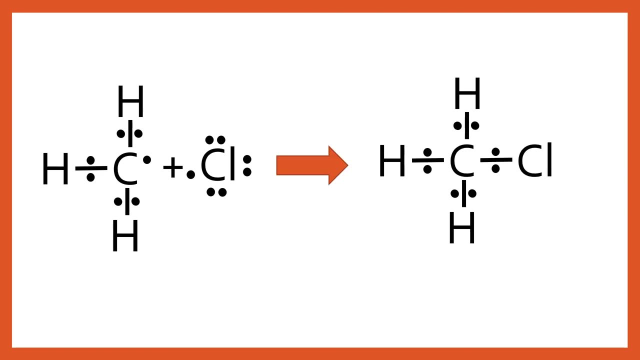 And that is going to solve some of the problem, And it soaks up two of the radicals and is, of course, a termination step. for that reason, What you could also see happening is a CH3 radical and a chlorine radical, And when they form together, you're simply going to get your. 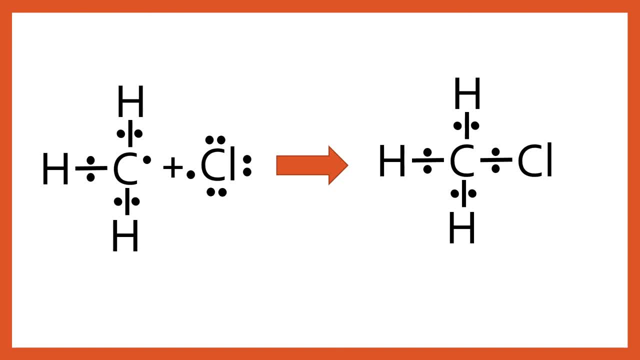 desired product, your halo alkane that you want to make in the first place, And so this reaction could simply be represented as so just showing the radicals and the product. These are the main termination steps that you're going to get, So let's start and summarize. 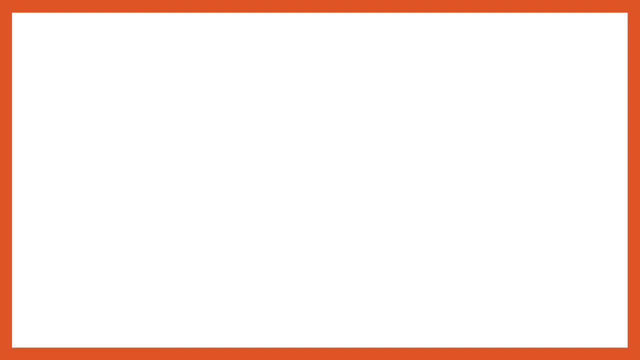 All of the reactions so far and get an overall picture of the key reactions that are happening and then look at a few of the side reactions that could also happen. So obviously we're going to start with the initiation step, and the initiation step is all about making those radicals to get things going. 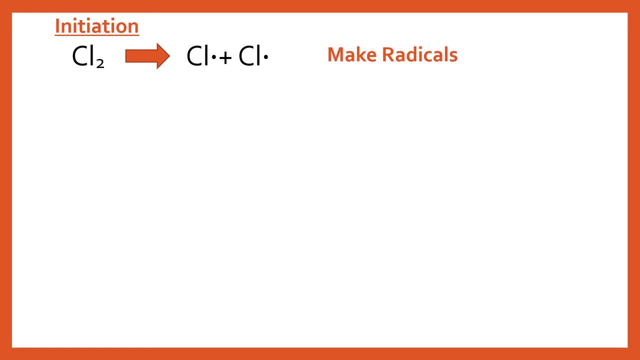 So you got the chlorine splitting up into two chlorine radicals. Then the propagation step. we have the chlorine radical actually reacting. So we have our CH4 finding a chlorine radical, forming another radical and a stable product, The radicals that's formed. then of course propagates the reaction. 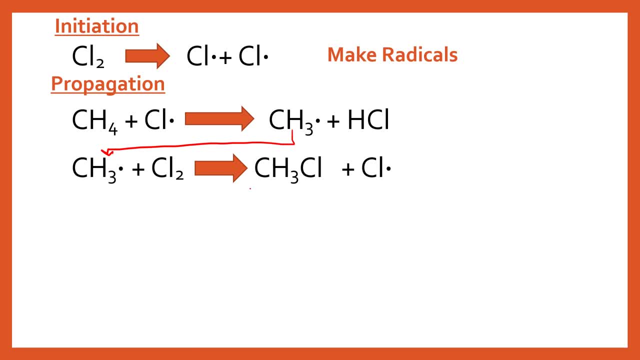 So we see this one's reacting with some Cl2 forming the desired product, but then also giving rise to a radical, And that radical could perhaps find the CH4 or it could do some alternative reactions, and the side reactions are things that we're going to look at in the next slide. 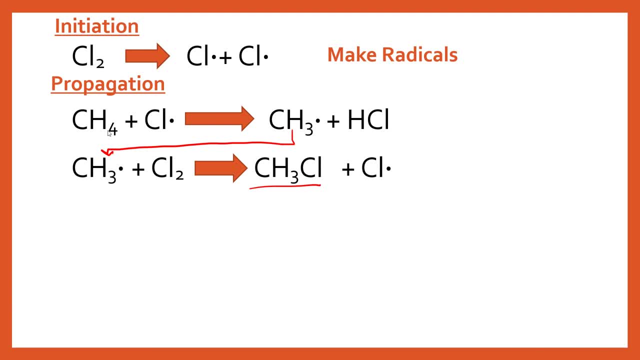 So we can also have a general way of expressing the propagation step. So the propagation step, we have a radical and non-radical reacting to form, form another radical and another non-radical. So it's like it's kind of swapping around: You're always having one radical used up but forming another one again. 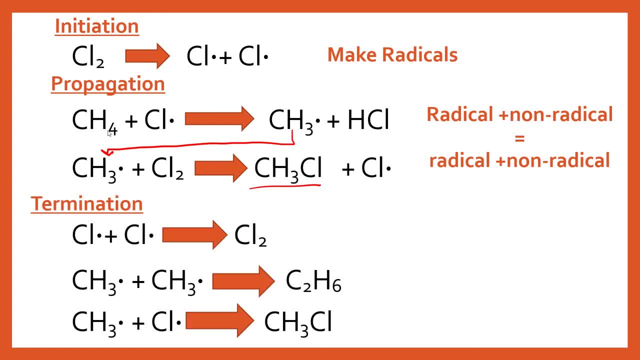 So you're propagating the reaction. for that reason, Then in termination we have various ways of soaking up those radicals and forming stable products that are not radicals, that are going to keep propagating the reaction. So the general rule for termination is where you have a radical and a radical reacting together to form a non-radical. 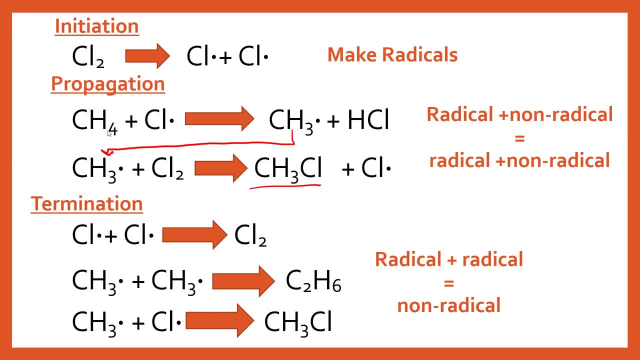 And that's putting a stop to the reaction. So this slide forms a nice summary of the principal reactions that are going on in the synthesis of this haloalkane. This isn't the only thing that's going on. I'm going to show you an example of a little side reaction that could also be. 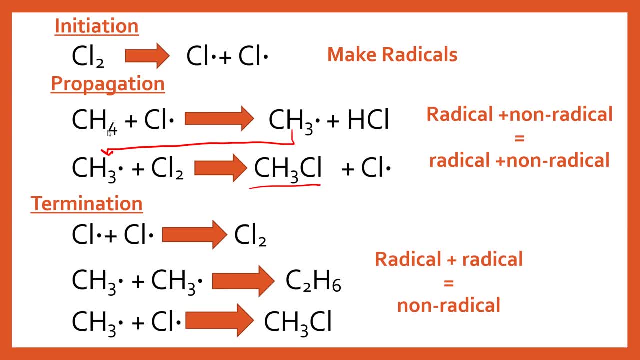 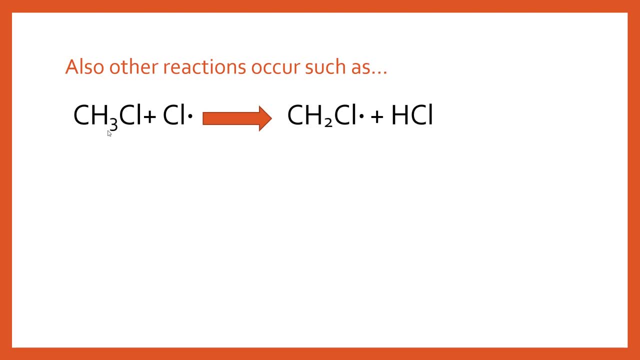 happening and one of the reasons why this isn't the best way to synthesize haloalkanes. So we've got some other reactions that could occur, such as this one where our chlorine radical forms a new product with our product, And so you're ending up with the CH3 dropping down to CH2.. 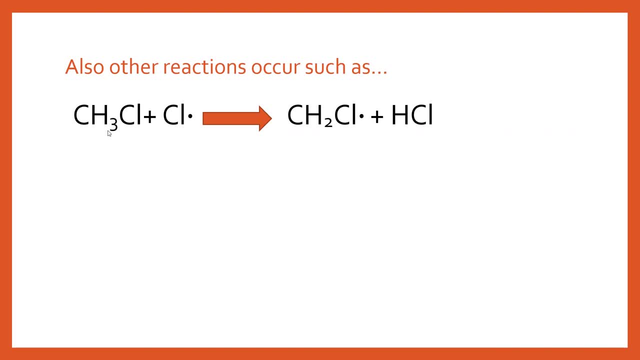 And one of the hydrogens is being replaced by a chlorine radical And you're also getting some more HCl, Then what could happen is that this radical could react with a Cl2 and you could end up with CH2Cl2 and you're now getting a different product.